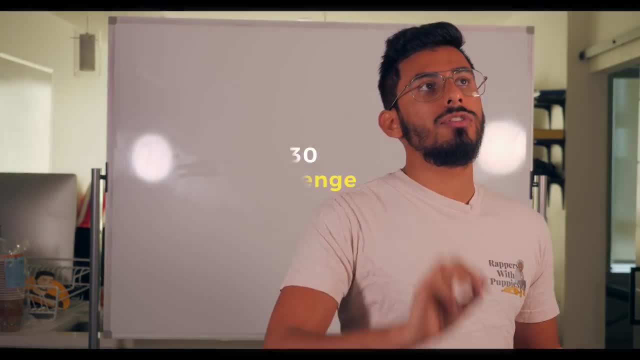 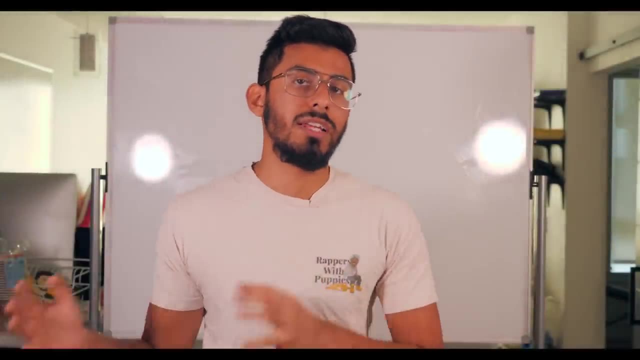 understand it. I made a video yesterday. Oh, by the way, this is also day four of my video challenge, So I'm doing the 30 days of videos, one video a day. So if you want to do some kind of challenge, 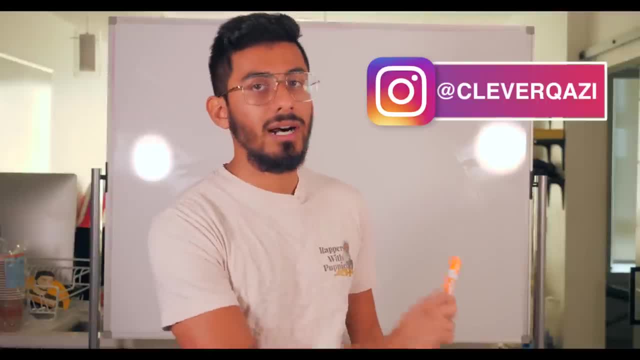 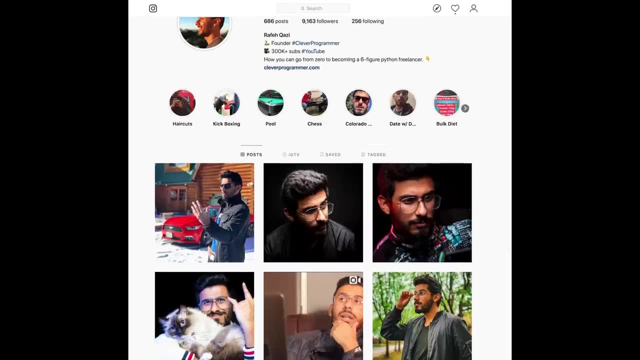 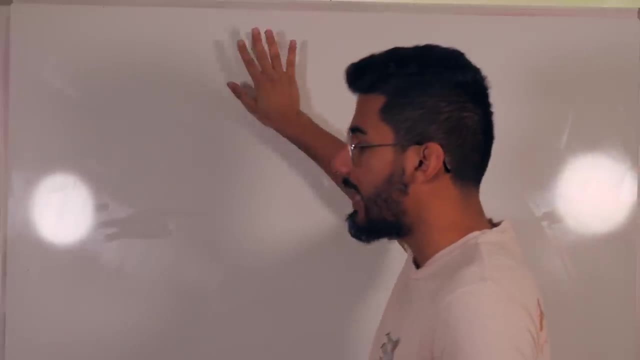 do it with me, And you can also follow me on Instagram. Clever Kazi And I am a lot more active on my Instagram And you can also follow me along and see everything that I'm doing, including the challenges in my routine. But back to the video. So how do you think about your? 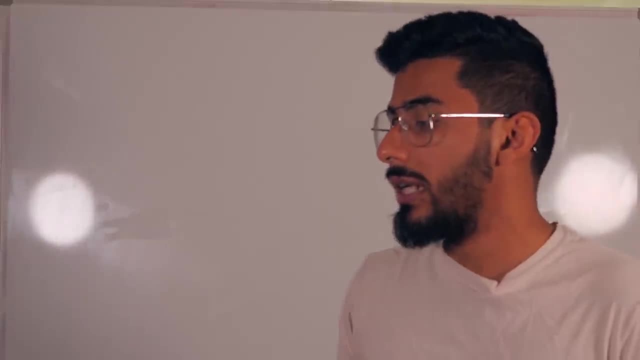 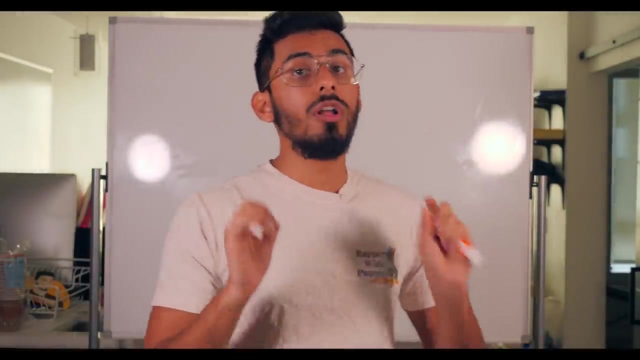 problems effectively and how do you actually improve? So in my previous video I talked about what are the effective tips to learn how to code. all right, And that was also really amazing. I'm going to pop that up right here. But in this video I want to talk to you about how can you? 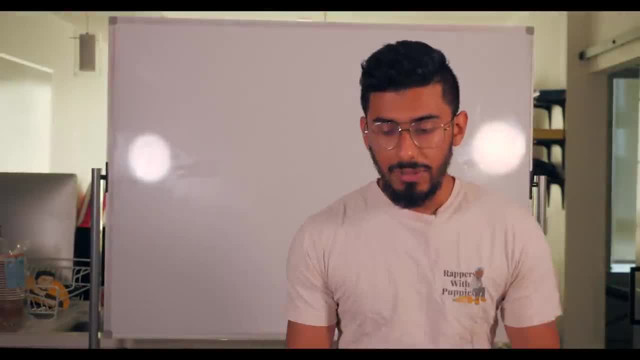 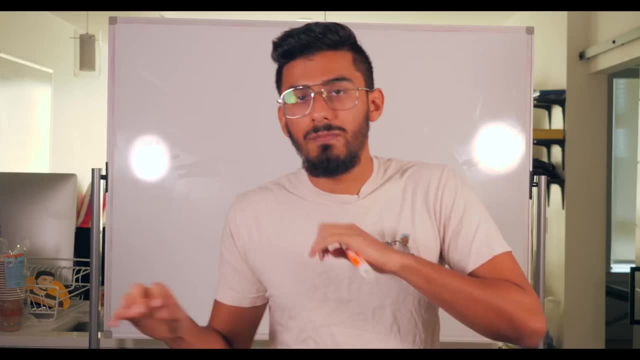 actually think about solving problems. So let's say you have some kind of problem, What do most people do? They just start writing code, especially beginners. They just start writing code and they try and see if something works. If something doesn't work, they just write more code print. 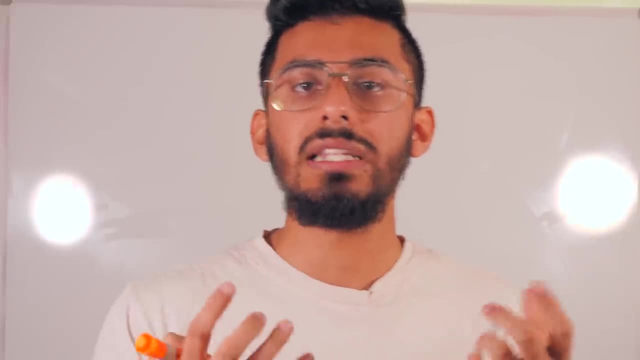 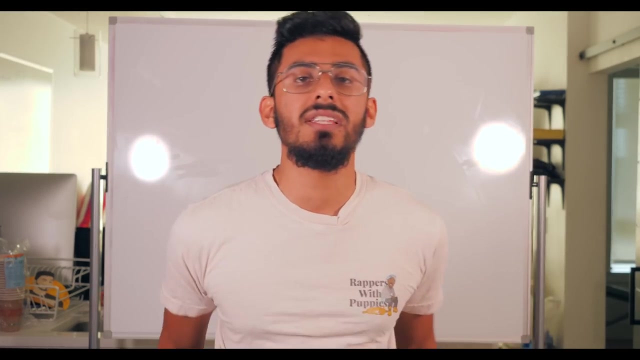 more stuff, But they're thinking about the program very, very lightly And they're thinking about the program very linearly. It's this one thing. So let's say you have to make- I'm going to use a simple example- Let's say you have to make a tic-tac-toe game. If they have to make a tic-tac-toe, 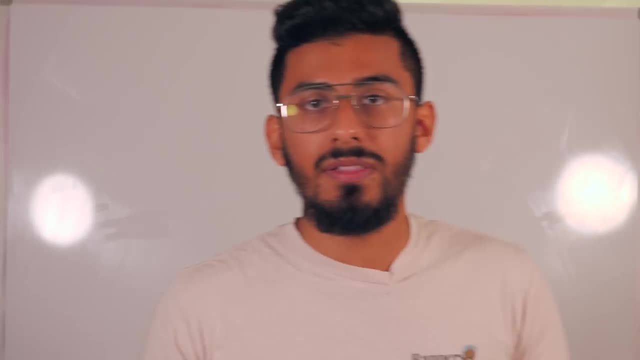 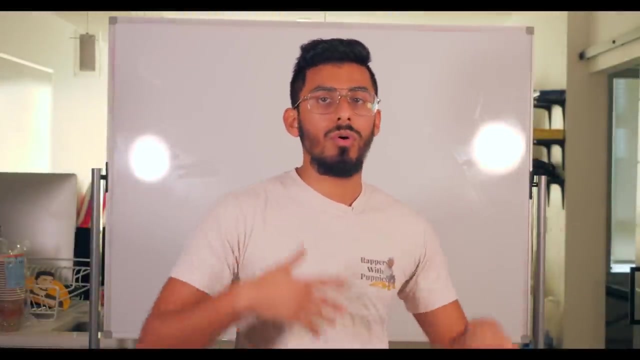 game. they'll just start writing it And they will think of everything as just one thing. So this includes, you know, they'll think of the diagonals and the columns and the rows and all that as like one thing and they start coding something up. But what you actually need to do before you start on, 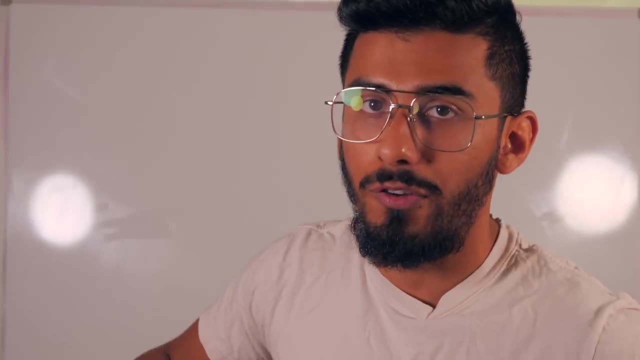 this is: use a freaking whiteboard. Whiteboards are awesome, so get a whiteboard. if you don't have one, Invest in one. It's one of the best investments you can make. But if you don't have a whiteboard, just 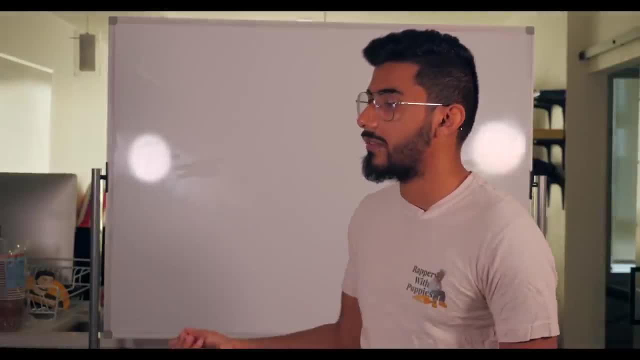 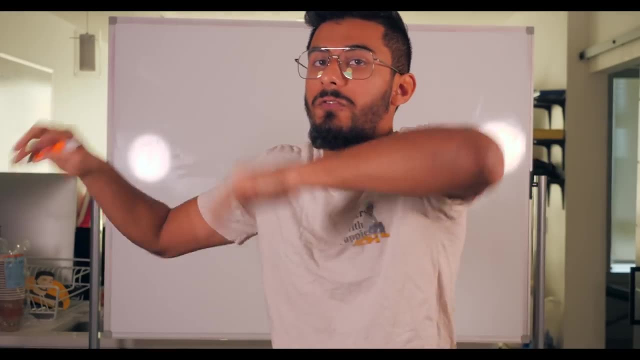 use a piece of paper or something, okay, But you want to think about this problem And coding is thinking, And I feel that sometimes people forget that When they're following tutorials, they're just typing stuff and following along. They're not actually actively thinking When they are trying. 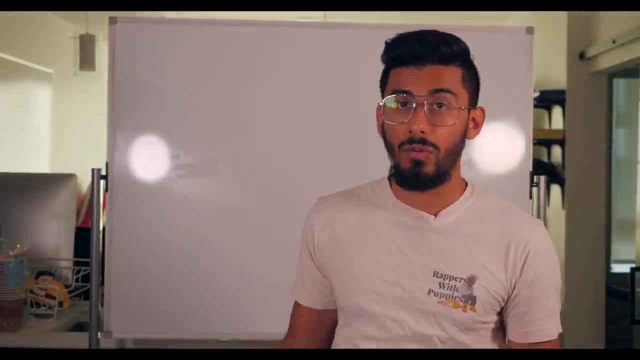 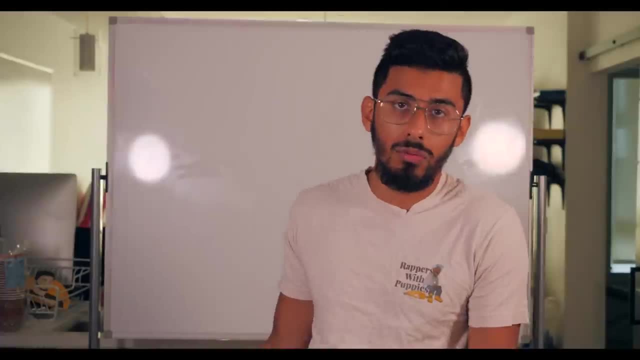 to solve a problem. they're just like typing stuff, running it in the terminal and see if it works. But if you want to go about solving a problem, you need to think about it. So if you want to go about solving a problem, So if I have to solve a problem like the tic-tac-toe, right, I'm going to be. 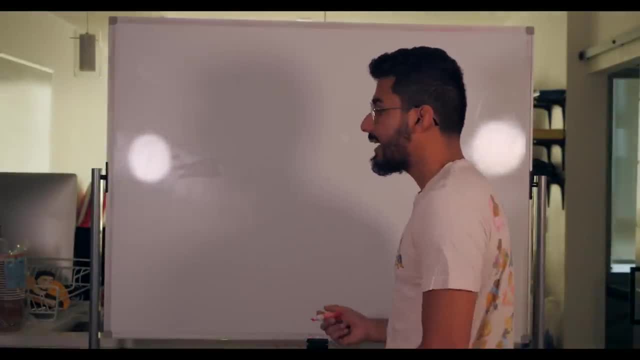 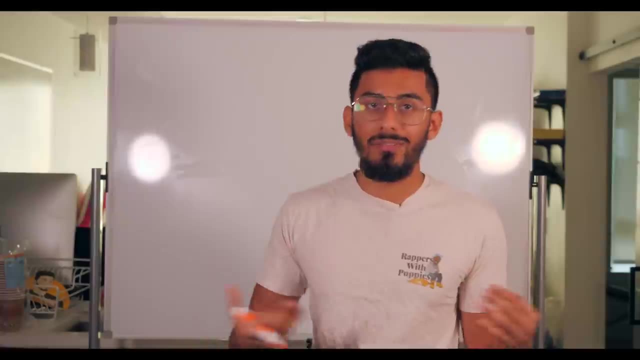 thinking about. I'm going to break it up into different components. So tic-tac-toe, first of all, tic-tac-toe, I have to come up with a representation of the grid of the board. So first I'm going to 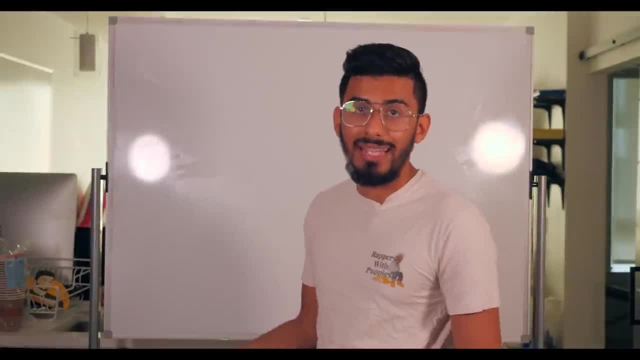 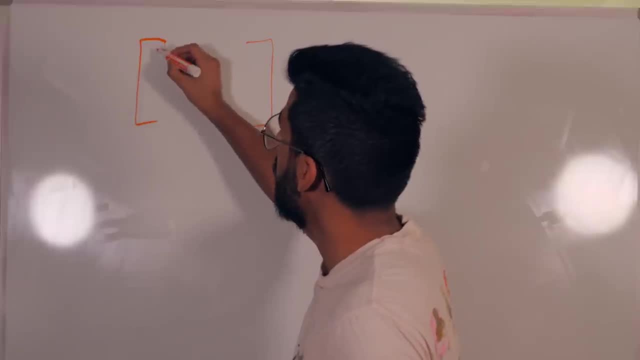 be like: okay, first, the thing I would have to do is actually create a board, right, A three-by-three board. So you know, that might be like this type of board. okay And whatever. For now I'm just going to have all x's in there or all zeros or ones, doesn't matter. 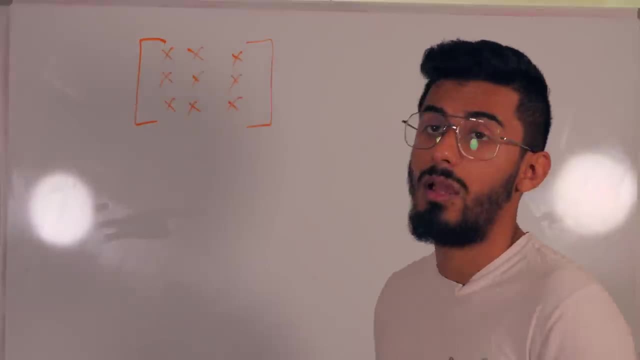 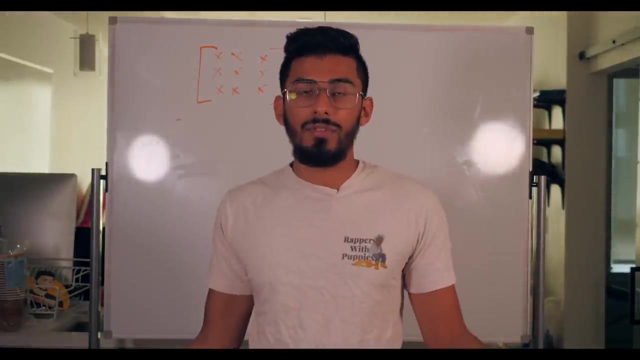 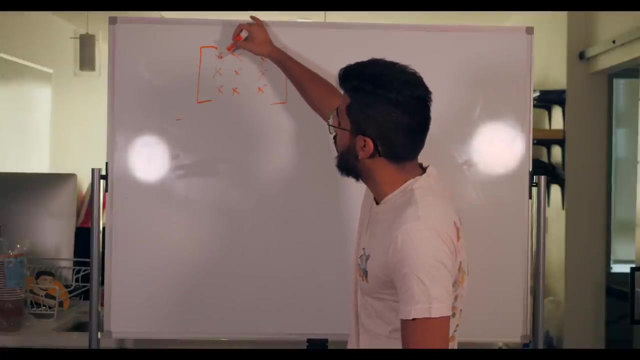 But first I have to represent this. This is my first problem. Then my second thing is that: how do you detect a win? So I need to be able to detect a win. So what are some ways you can detect a win? Well, okay, I can detect a win based on rows. So if you have all three in a row, you can win. 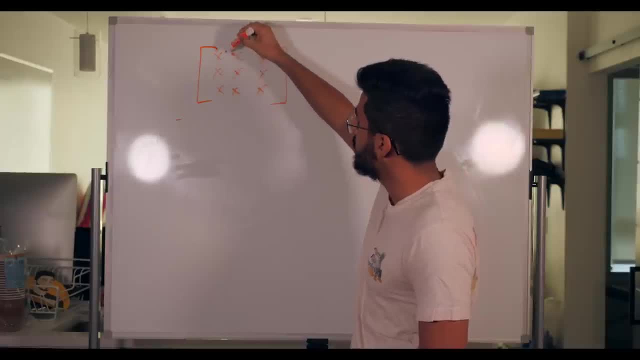 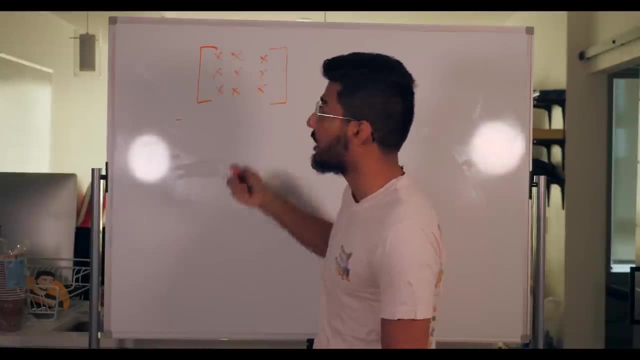 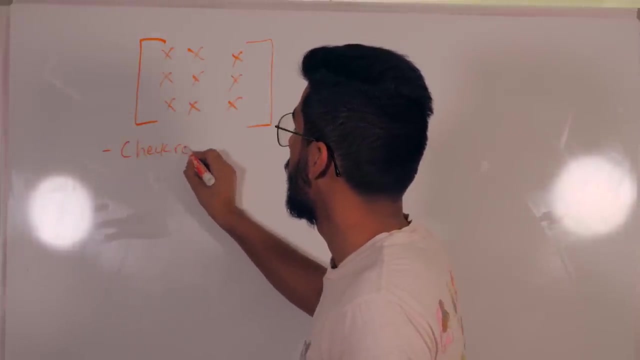 Right, And you have to check consecutively. Then I have to detect a win on the columns, and then I have to detect a win on the diagonals. So that means that I'm going to create like a function and I'll have one function that'll just be called like check rows. Pretty simple, right? So I'll. 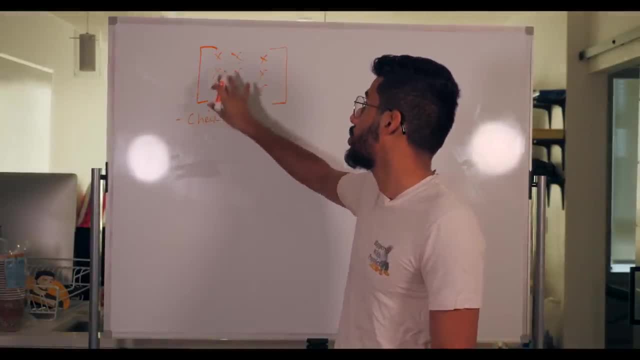 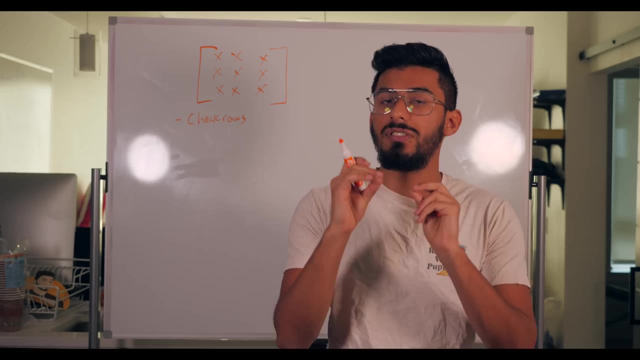 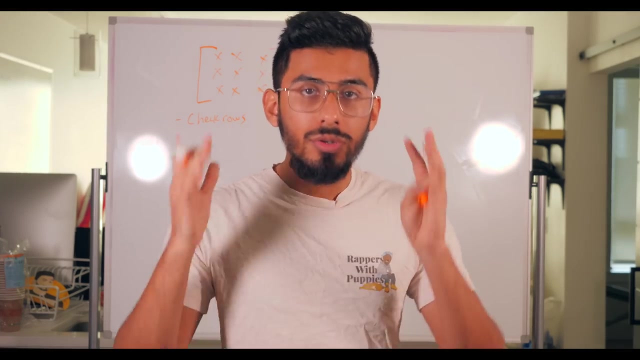 write one function and all that function's job is to check the rows. That's it. So what I'm doing is I'm taking this giant problem and breaking it into its component part. Taking this giant problem, it's almost like: how do you eat an elephant? How do you eat an elephant? You eat an elephant very. 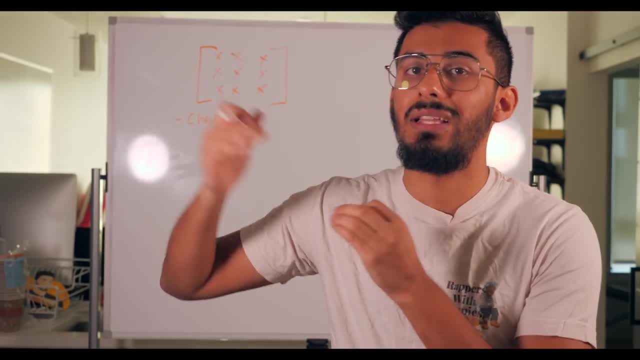 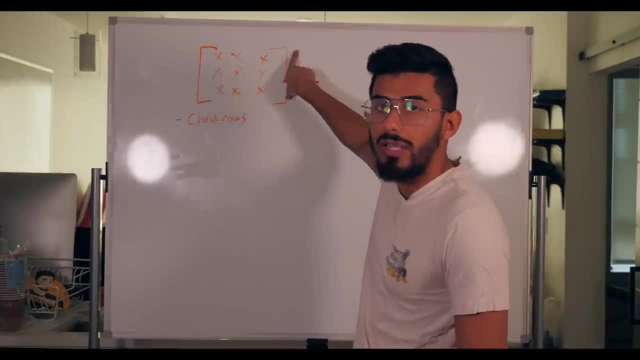 slowly and one bite at a time and over the course of days, weeks and months. I never ate an elephant, but I assume that's how you would eat one. Probably can't eat one in one sitting. Most people code like they're trying to eat the elephant in one sitting. It's not going to happen, You have. 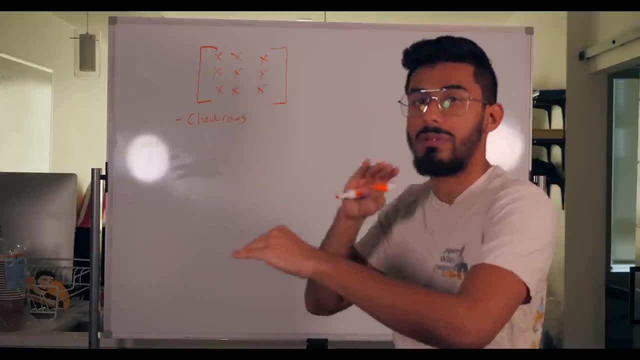 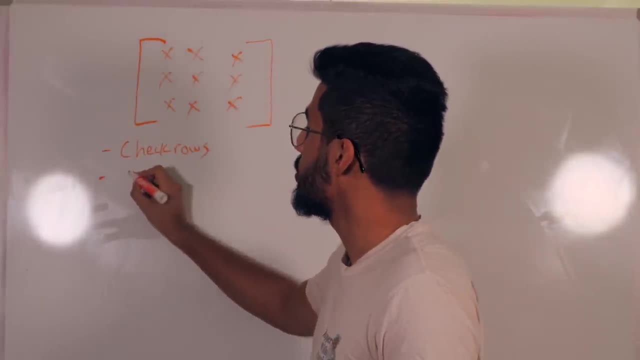 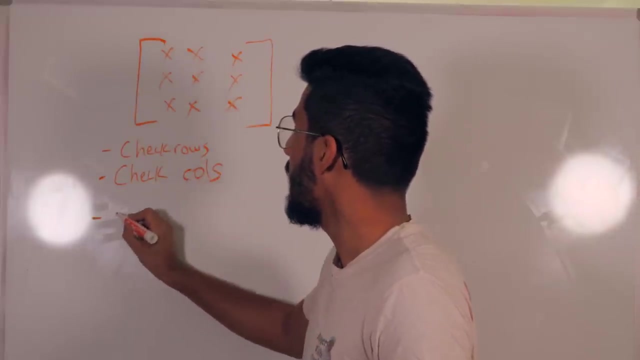 to break it down, You have to understand all of the component problems that one problem has. Right, It's a layer of problems. So I want to be able to check the rows, Then I want to create a function called check- let's say columns, All right, And then I'll create a function called check. 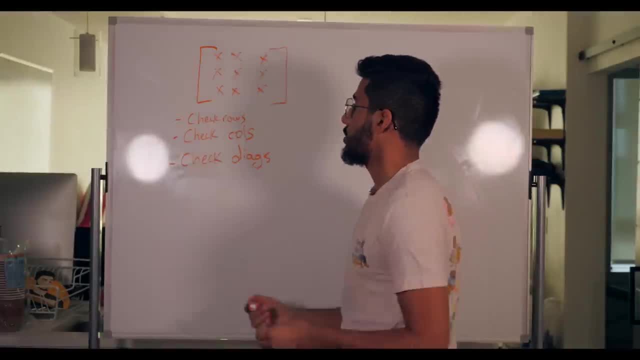 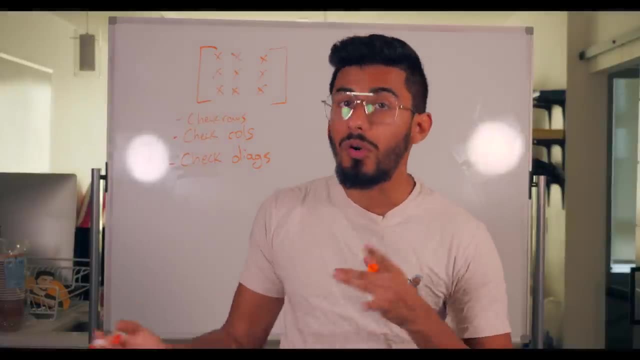 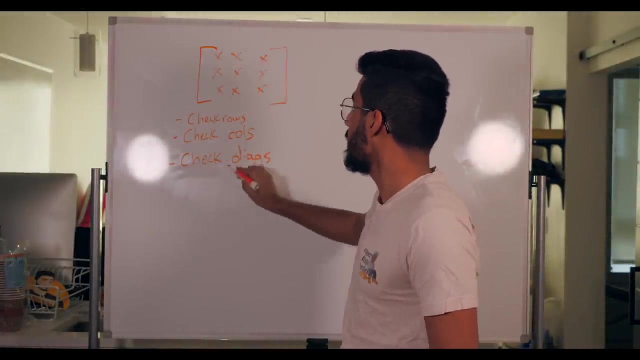 diags. So now I'll have three different functions. One function can check a row and tell you whether there's a win- somebody has won or not. Then we have a function called check columns and that is one on the columns or not. Then we can have check diags that can check if somebody's won on the. 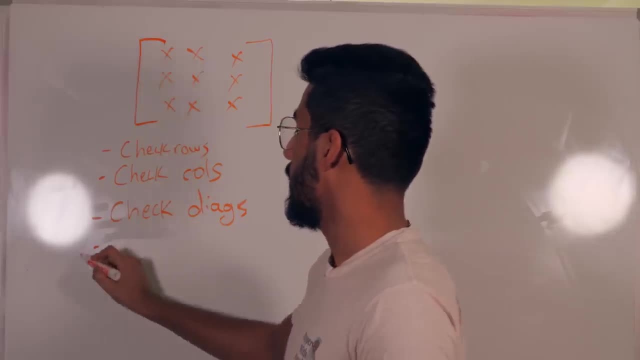 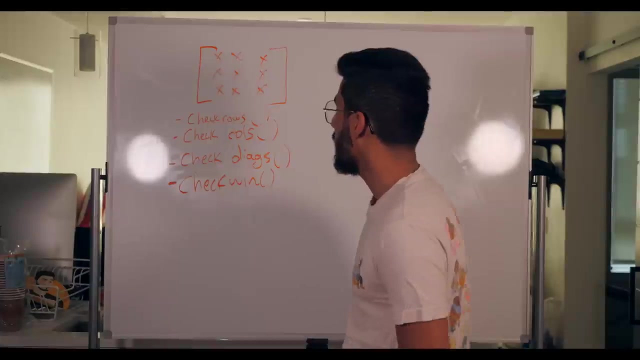 diagonal or not, And then we can have something called, you know, check win. All right, So we have all these functions, The check win function. well, all this can be, it can be just comprised of all three of these functions, right, Because you can just run check win and then it'll run check rows. 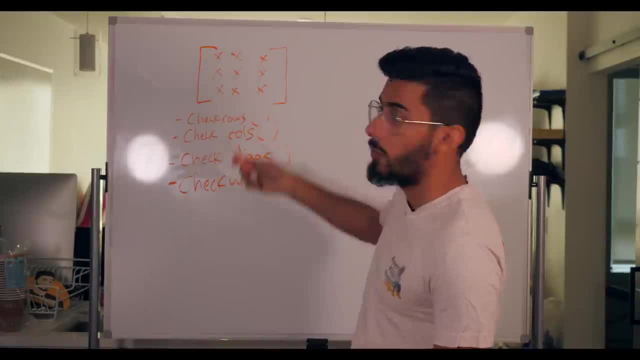 check diags and it'll run all three of these functions until it finds a win, All right. So right now we're just trying to think at a high level. We're not trying to get too bogged down in the coding details of how. 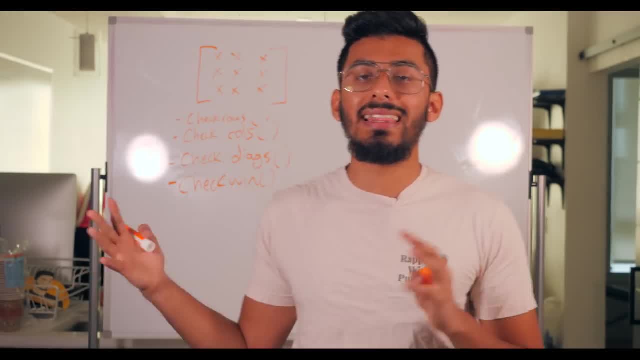 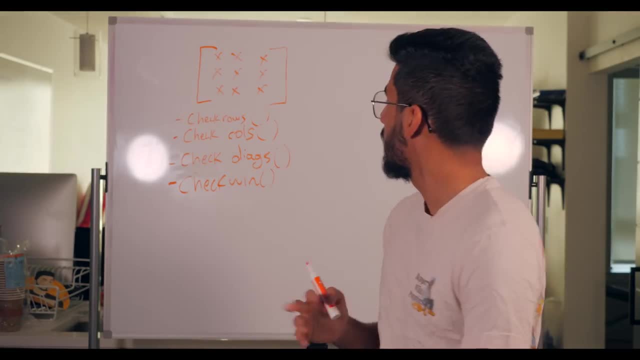 it's going to work, what data structure we're using. We're trying not to think about all those things. We're just trying to think at a high level of this problem and trying to solve it. you know, in these basic components, Eventually you'll have this to-do list and then all you do. then the part is easy. 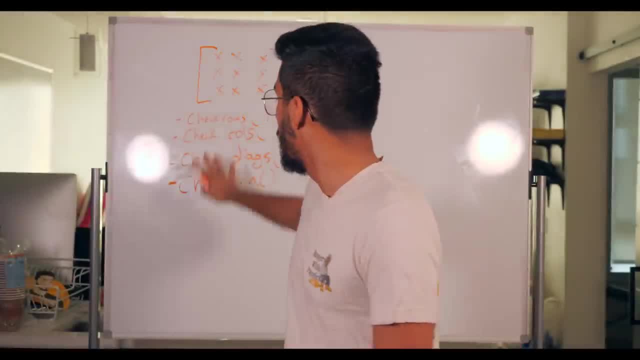 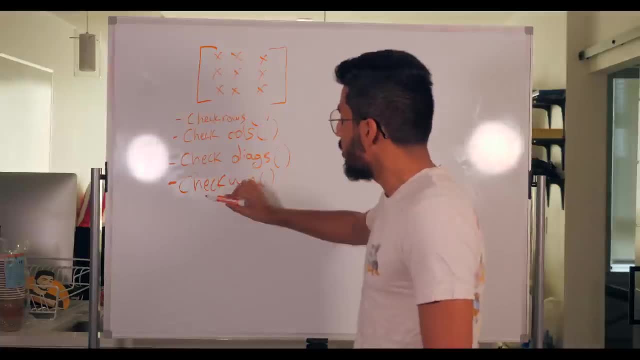 You write code, you do research, you figure out technically, but now you have a big goal of what you need to actually do, Because otherwise most of the people you know are coding blindly. I have all these functions that can tell me if a win took place right, And then I can have functions that can: 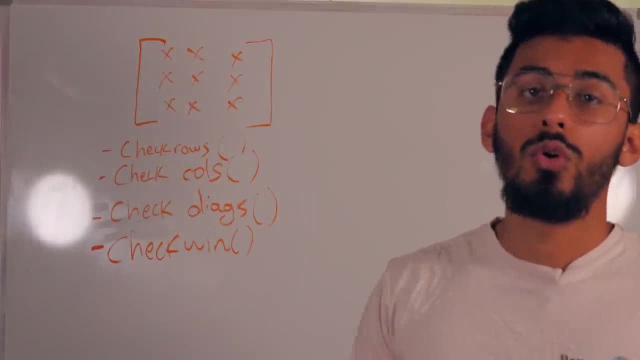 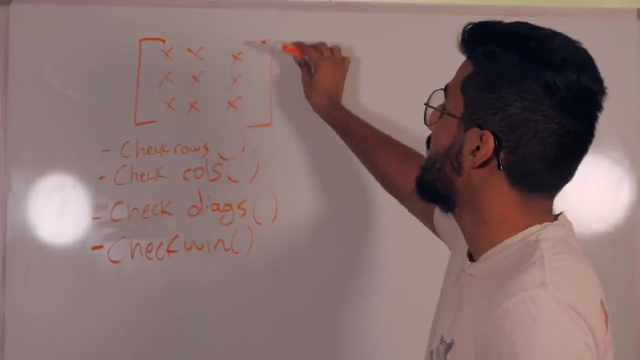 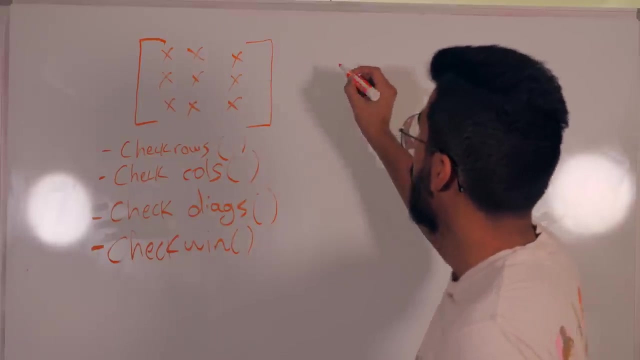 determine a loss. We can have a function that can detect whose turn it is or whether it's nobody's turn, right? So we need- we need some states as well for this board. We need to have a state where it tells us whether the game is still playing. So, for example, we can have a. 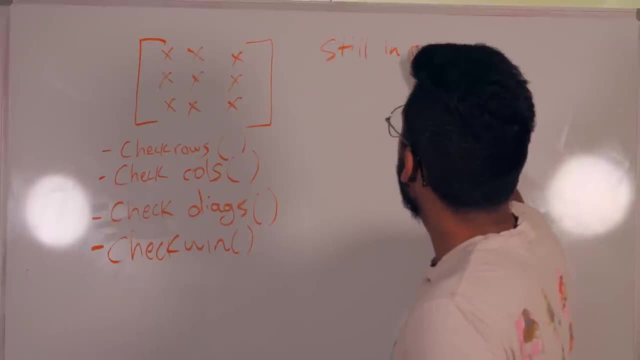 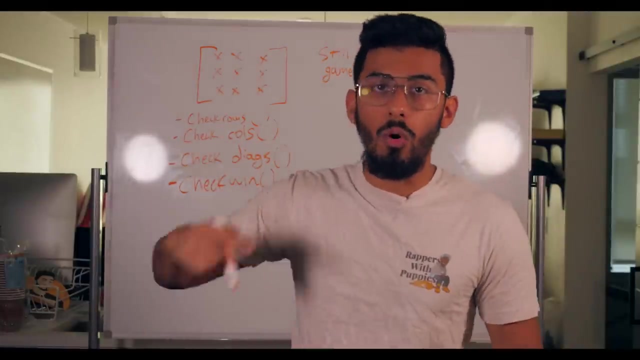 still in play or we can have a state that says, um, you know, the game is game over, So meaning somebody won. So what this would do is if we have a while loop right And we're running this game over and over and over again, then it would be in this state still. it'll always check if the game 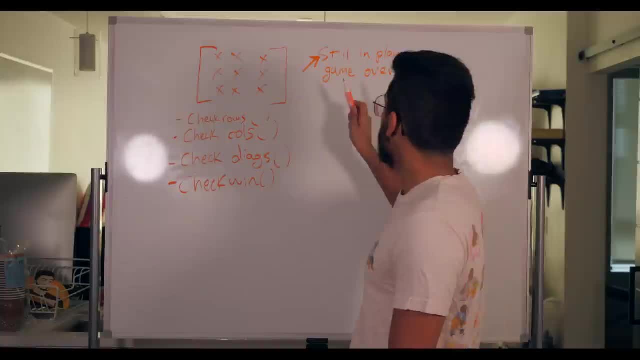 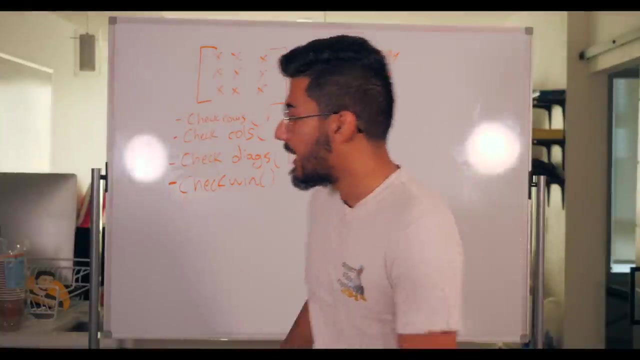 is still in play. But if the game is not still in play and somebody has won and somebody is connected- all three on either rows, columns and diags- it'll change the state of the game to game over and then it'll stop the game right, And then a new game might start after that. The point is not. 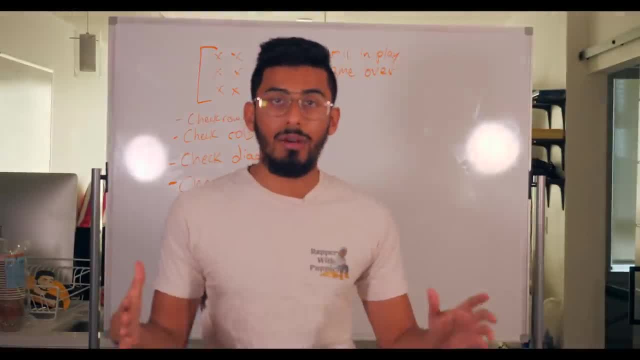 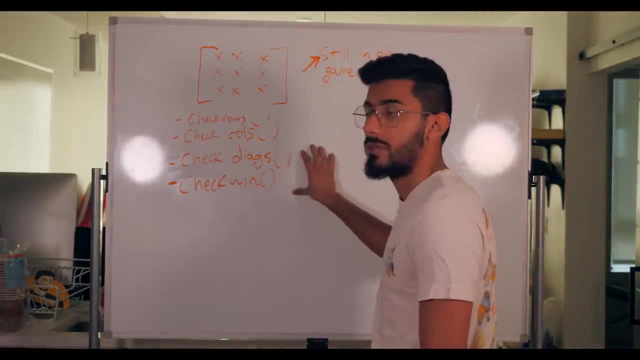 to solve this complete like tic-tac-toe problem right here right now. But my point is to get you to actually think at a higher level about your coding problems. You need to break them down into components and in the start, is going to require you to understand it in English or whatever. 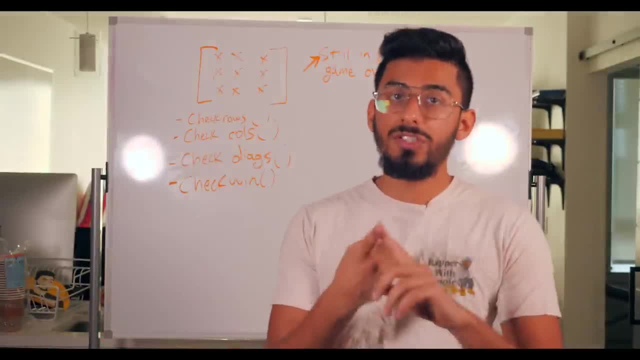 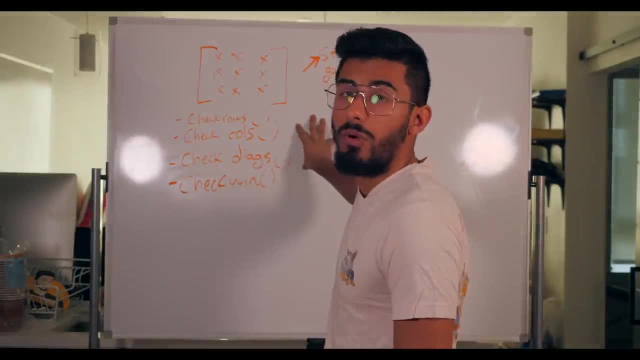 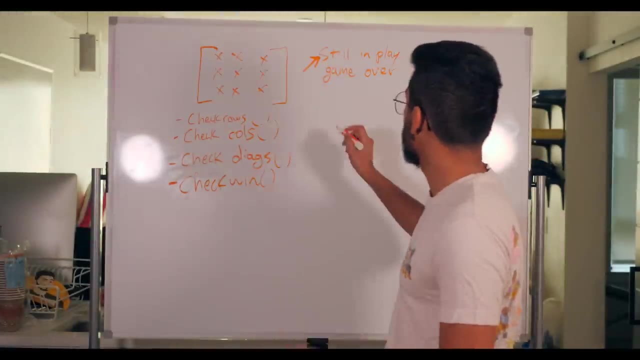 language is your, you know mother tongue. But first you're going to actually need to understand the problem in English and be able to describe it visually, have it somewhere. Then you need to break it down into its component parts and know exactly what you need to do. So first I will say: understand. 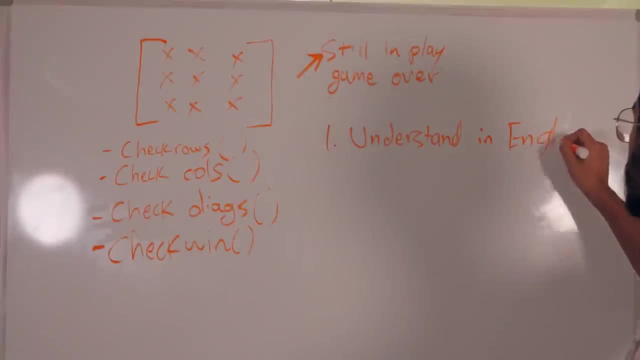 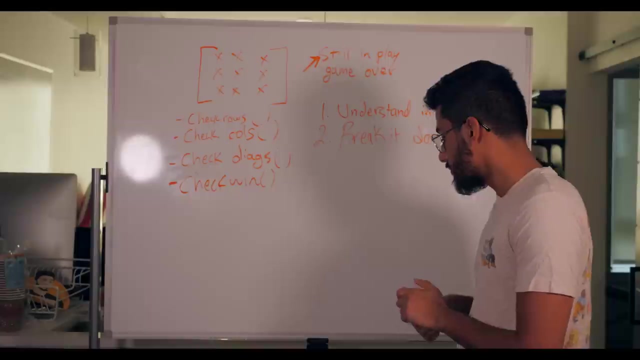 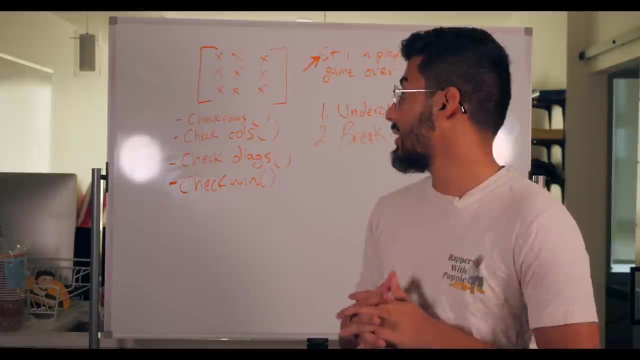 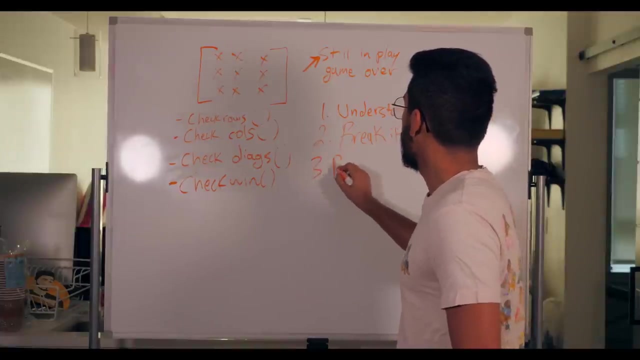 in English: Okay To break it down. Okay, So you want to break the problem down into its component parts. That way you know exactly what it is that you need to do, And then you have a plan of action. So after this, once you've broken it down, you know you're have a plan of action. 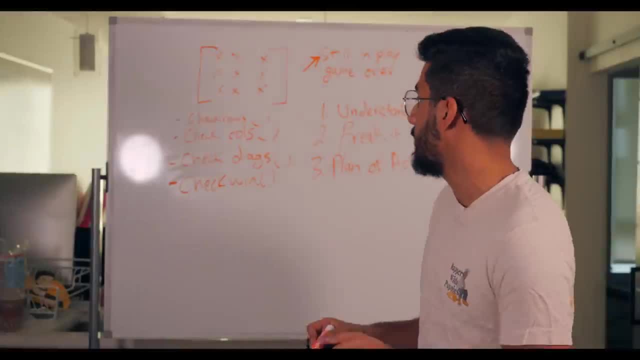 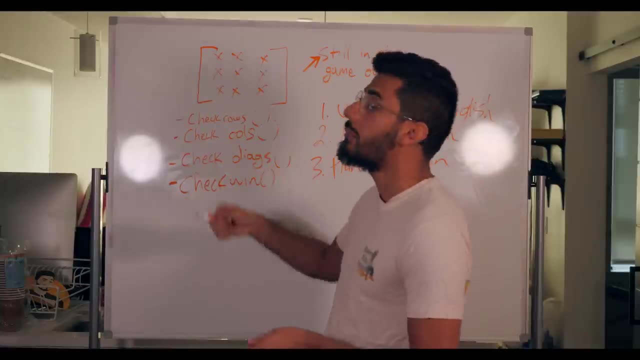 And then it's simply about what order you want to do this in. What's going to be like: are you going to make check rows first? Are you going to make check wing first? You're going to make check diags first, Or are you going to make the 3D board representation first? So it all is going to be about. 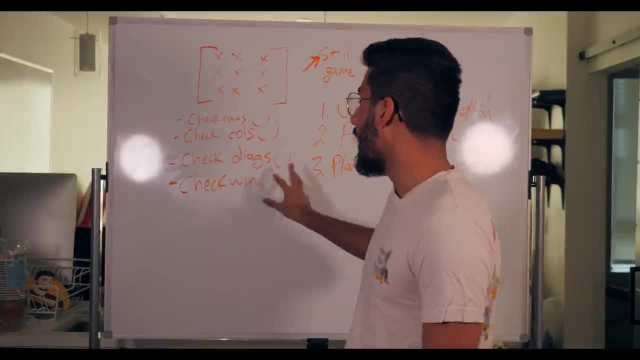 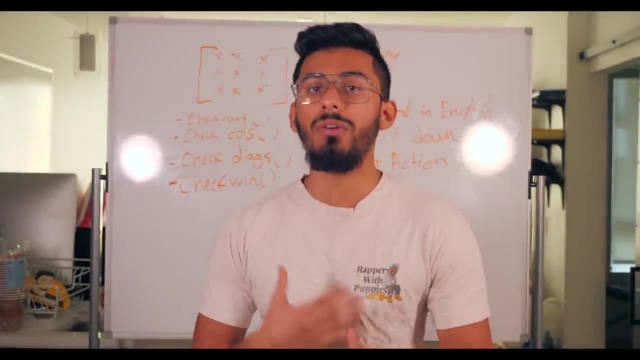 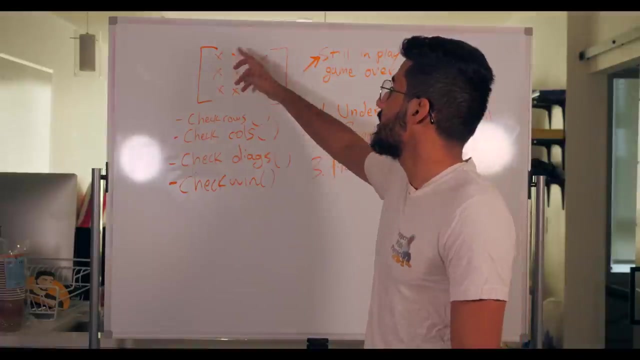 you know what your plan of action is And then, once you get inside of a function, that's when you start needing to worry about what data structure you'll be using, how you'll be actually making it happen. You know, for example, are you going to be using a dictionary or are you going to be using 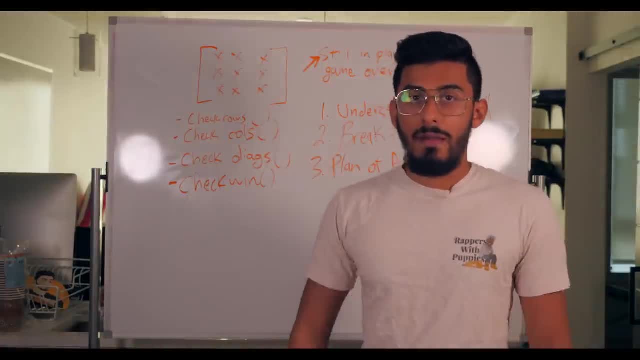 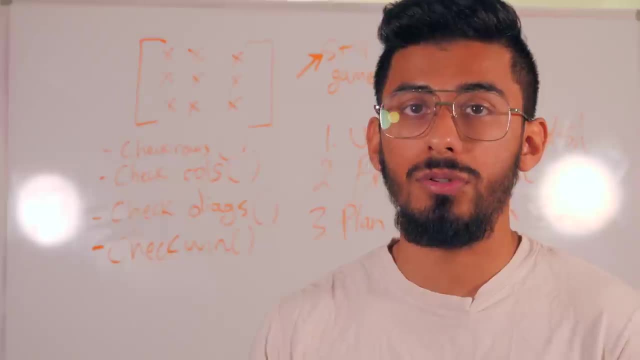 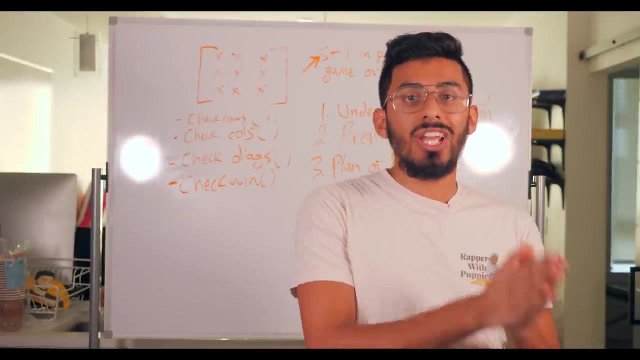 a list of lists to demonstrate a 2D board. Okay, So that those are the things that you're going to need to think about later. So hopefully this video has helped you or at least reminded you of some of things you might have even known. but now I encourage you- you know again- to do a daily